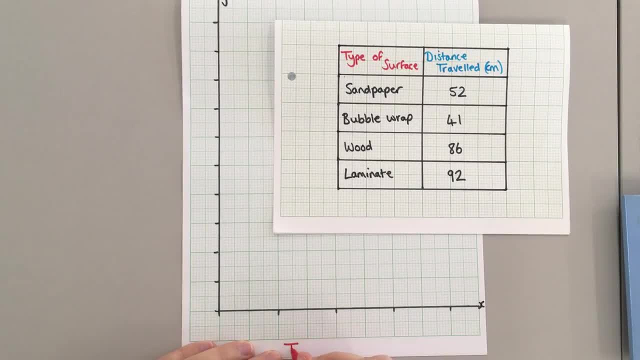 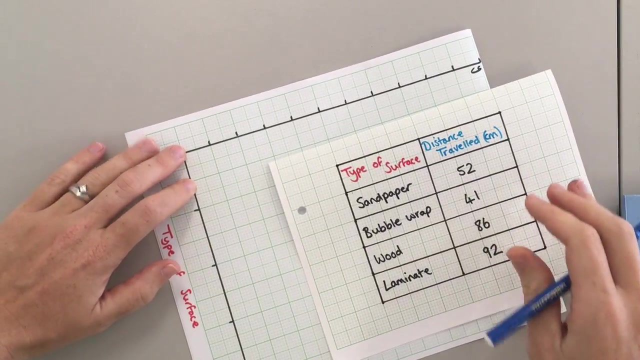 along the x-axis. So I'll label my x-axis with my independent variable, the variable I change the type of surface. There's no units for this. For the y-axis, we put the dependent variable found in the right hand column, the thing. 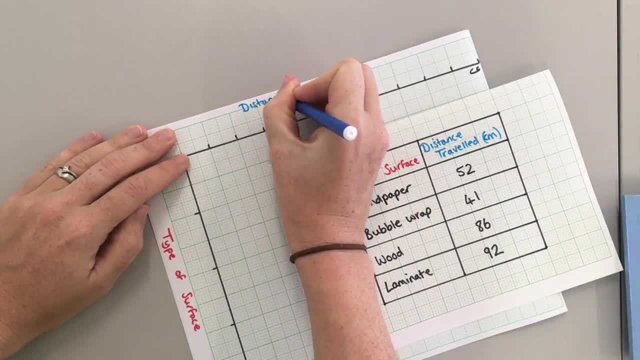 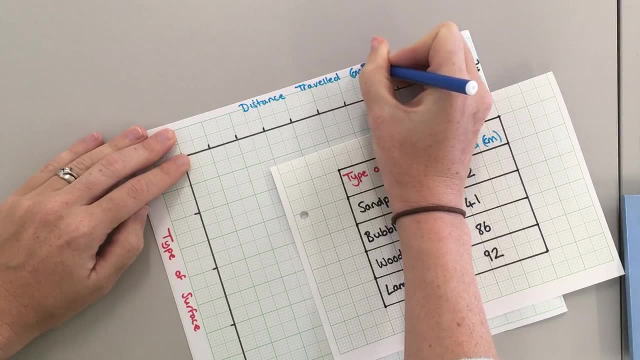 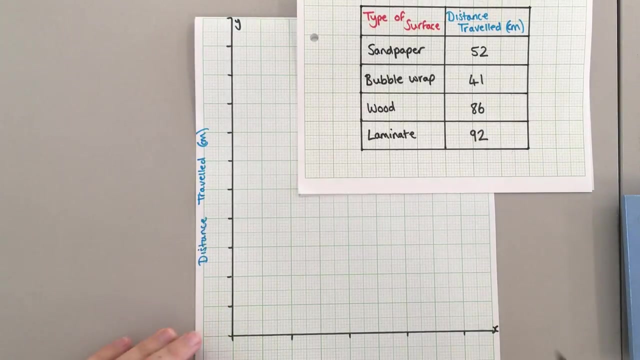 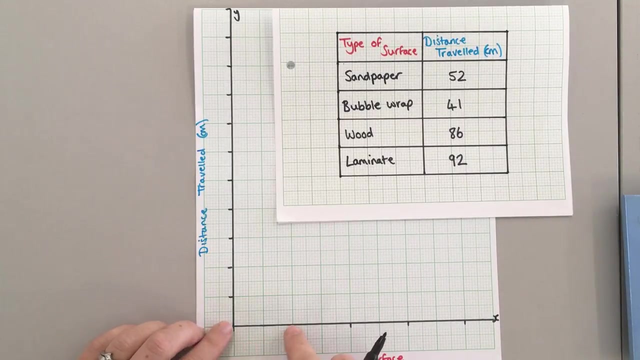 I'm measuring which is distance travelled, And the units are centimetres. Now I need to add some scales. So this is a bar graph, So I'm going to write my scale And then I'm going to add my labels in between these markers. 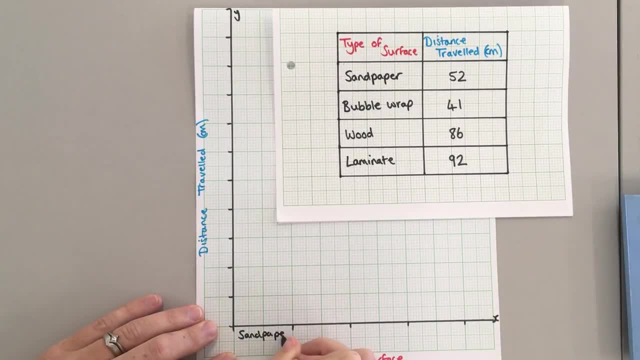 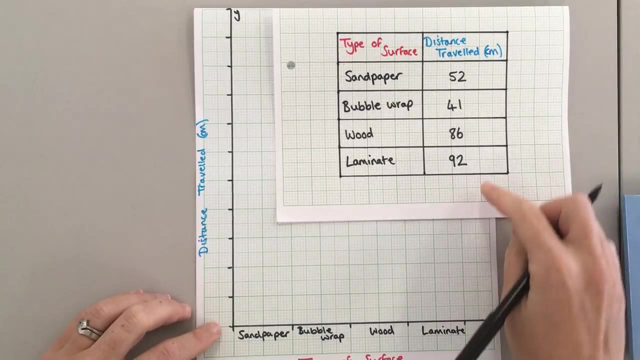 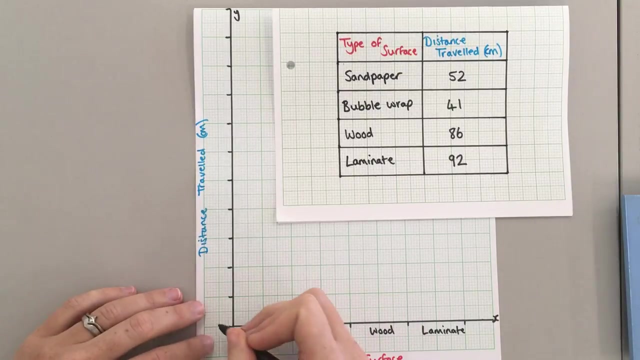 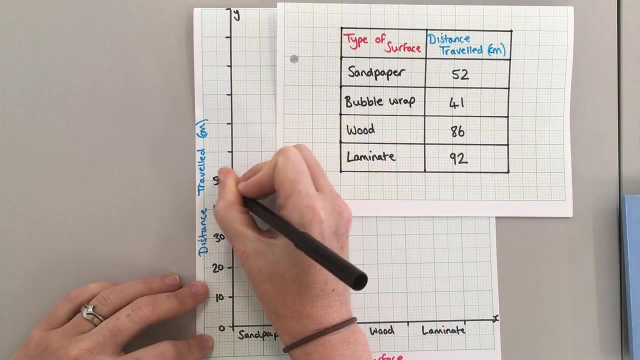 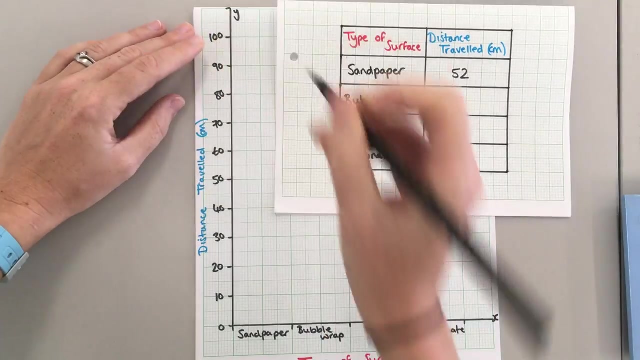 So I've got sandpaper, bubble, wrap wood and laminate Up the side. I need to get to 92.. So each of these gaps has 10 small squares. so it makes sense for me to go a bit faster. So I'll go up in tens: 10,, 20,, 30,, 40,, 50,, 60,, 70,, 80,, 90 and 100.. 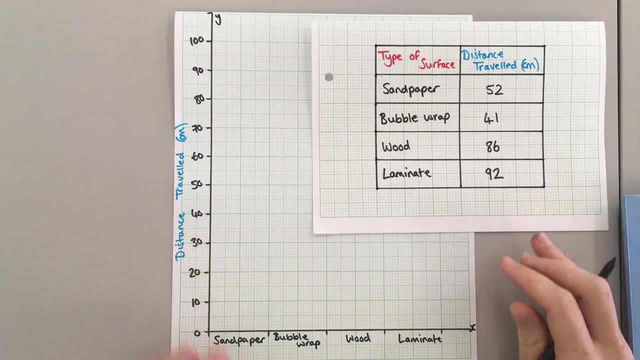 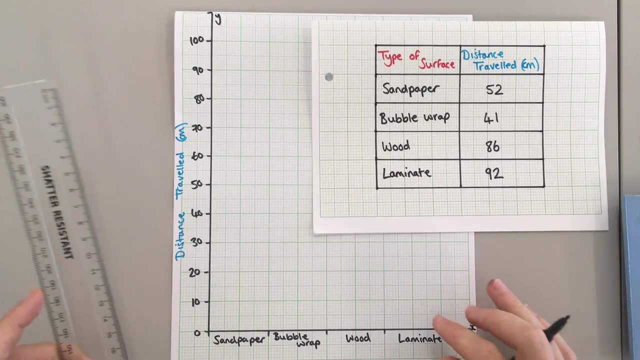 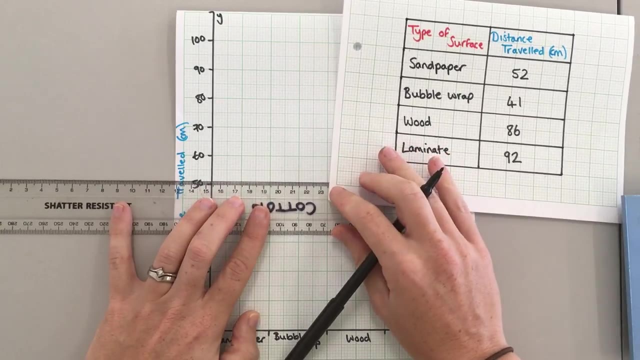 Then I'm going to plot my bars. You can have your bars touching. That's absolutely fine. Please use a ruler. So sandpaper goes up to 52.. So 50, one tooogs. Each of those small ones counts as one. 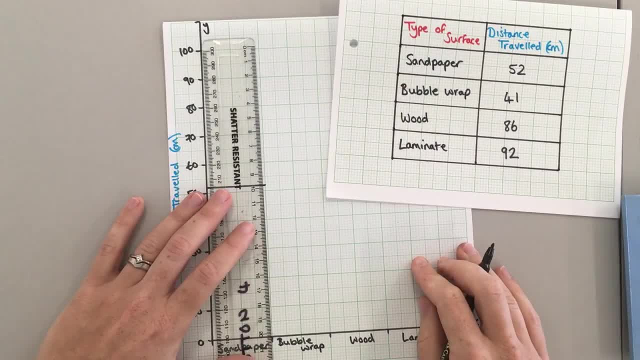 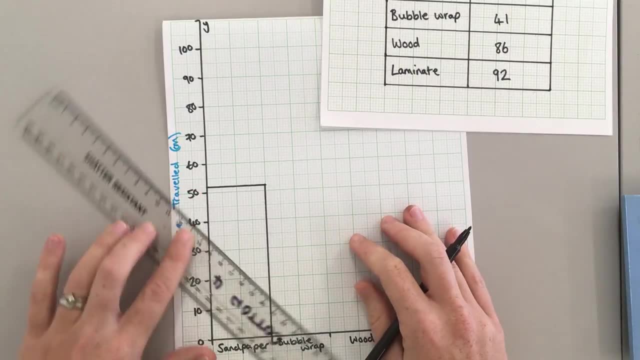 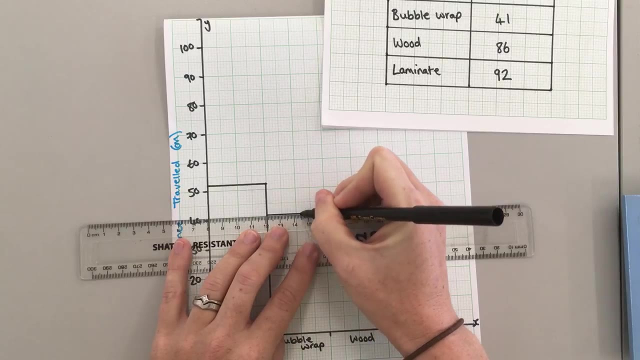 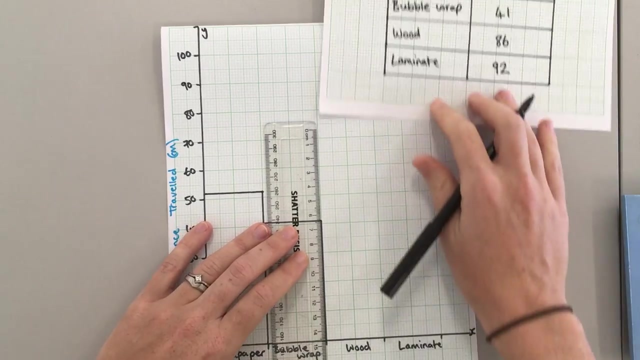 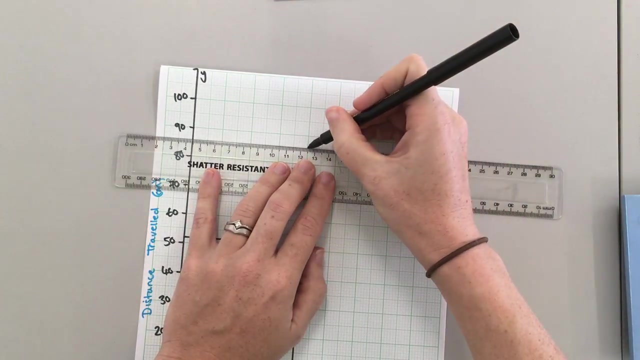 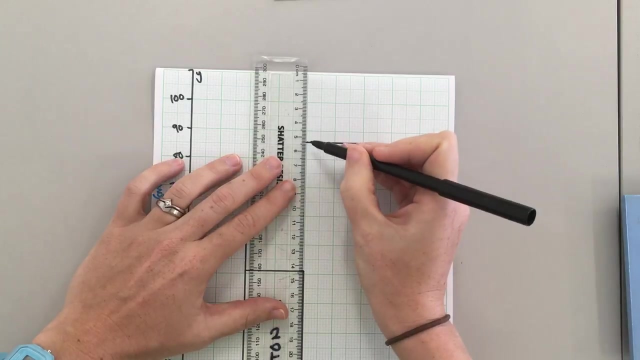 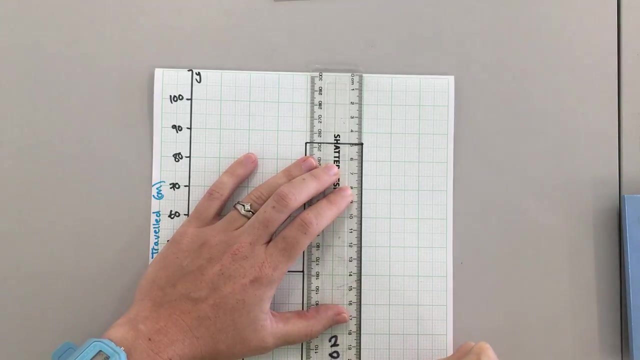 So I draw a line across and then I'll join it up to the bottom, like so For bubble wrap 41. So again I find 41. Draw a line across, Join it up to my x-axis. Wood went up to 86 and then laminate went up to 92.. 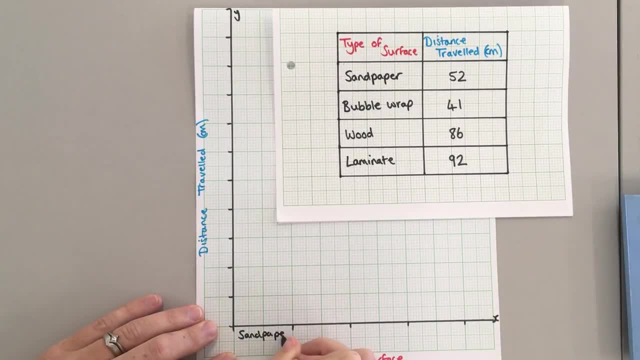 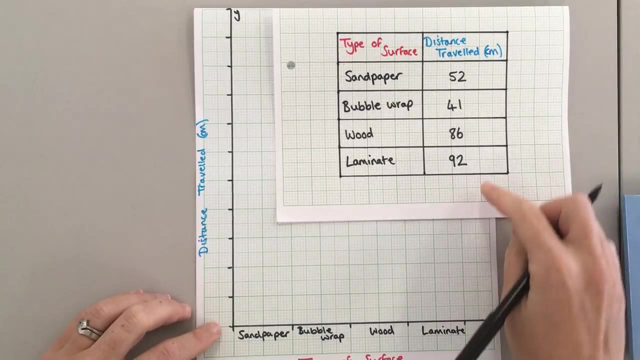 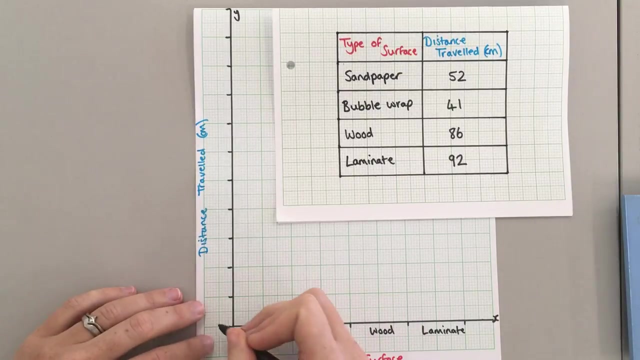 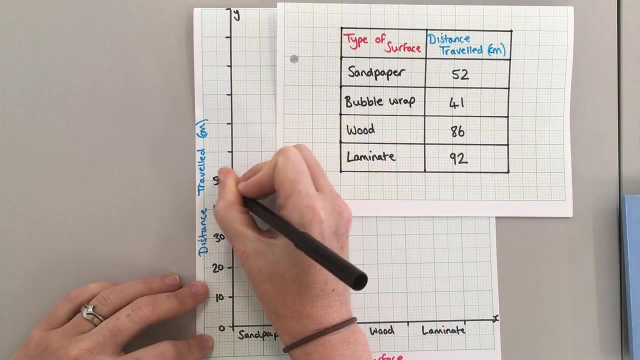 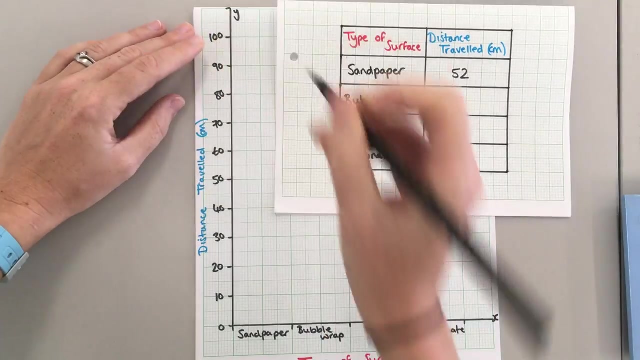 So I've got sandpaper, bubble, wrap wood and laminate Up the side. I need to get to 92.. So each of these gaps has 10 small squares. so it makes sense for me to go a bit faster. So I'll go up in tens: 10,, 20,, 30,, 40,, 50,, 60,, 70,, 80,, 90 and 100.. 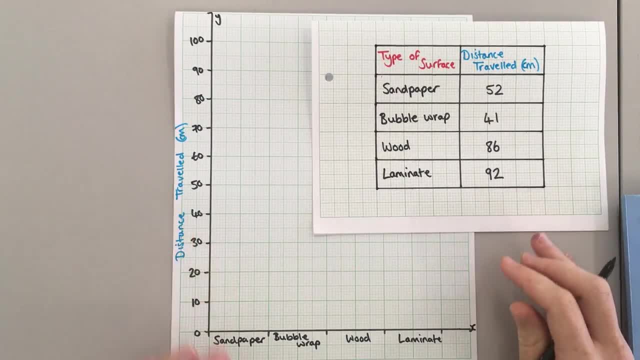 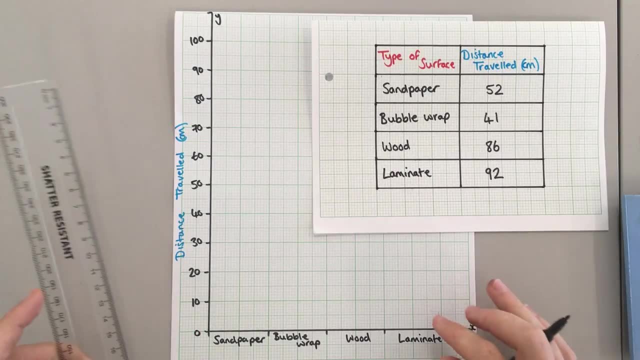 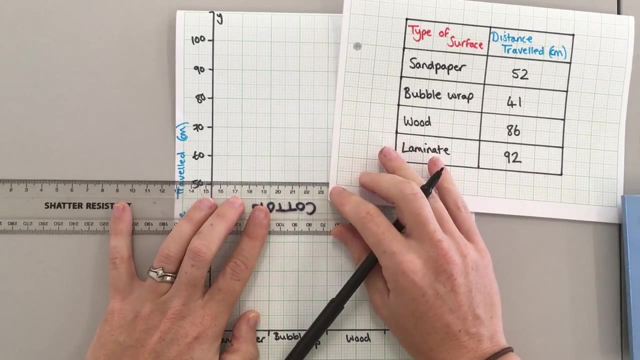 Then I'm going to plot my bars. You can have your bars touching. That's absolutely fine. Please use a ruler. So sandpaper goes up to 52. So 50, 12. Each of those small ones counts as 1.. 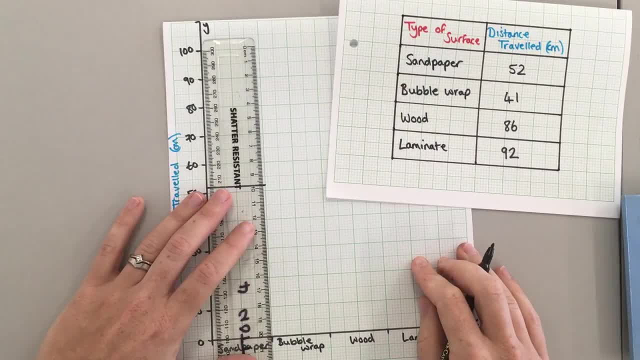 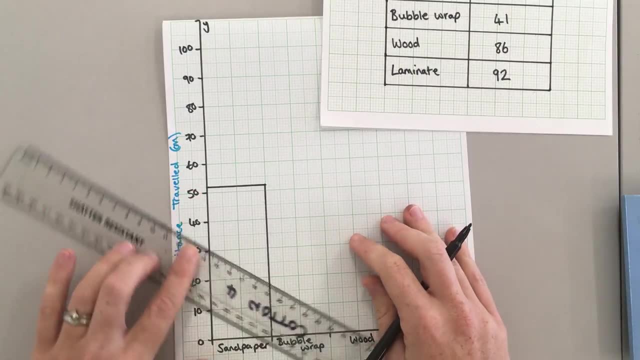 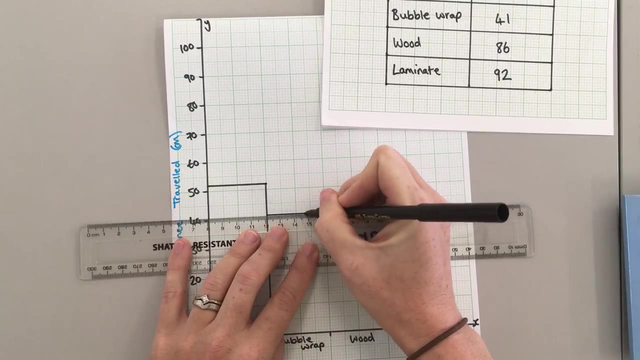 So I draw a line across and then I'll join it up to the bottom, like so For bubble wrap 41. So again I find 41. Draw a line across, join it up to my x-axis, Then I'll draw a line across. Draw a line across, join it up to my x-axis. 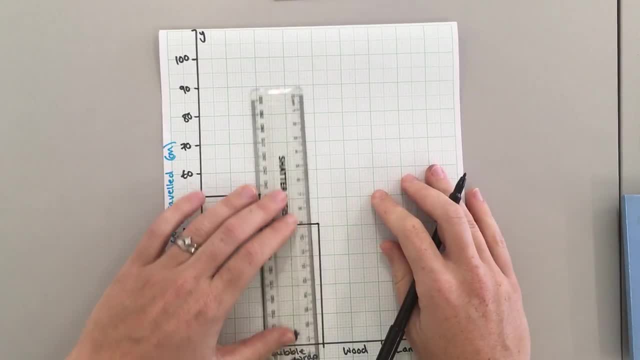 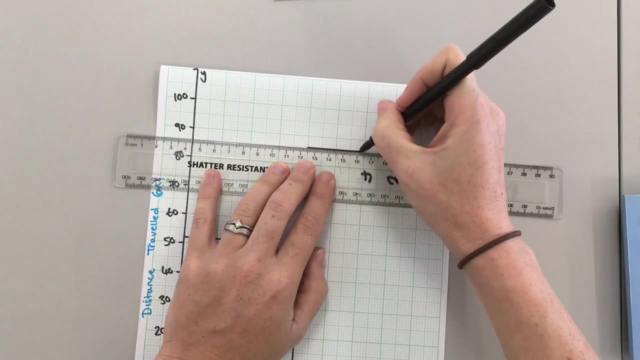 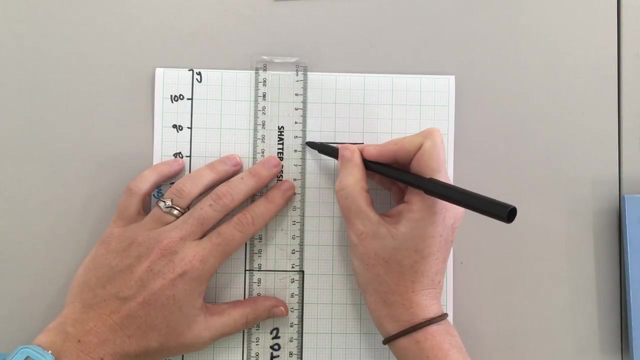 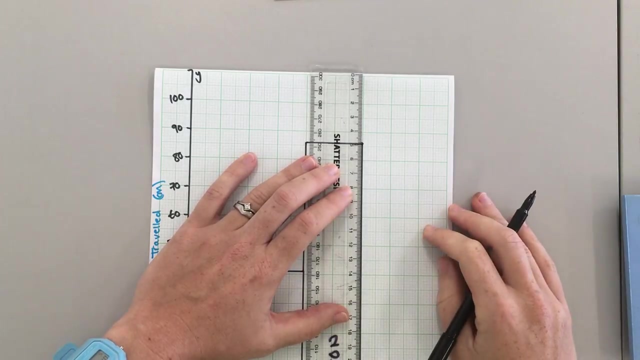 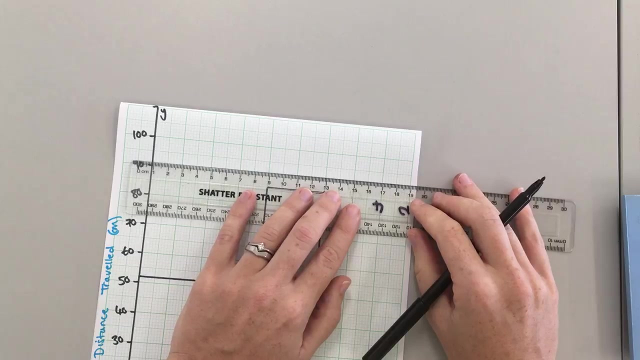 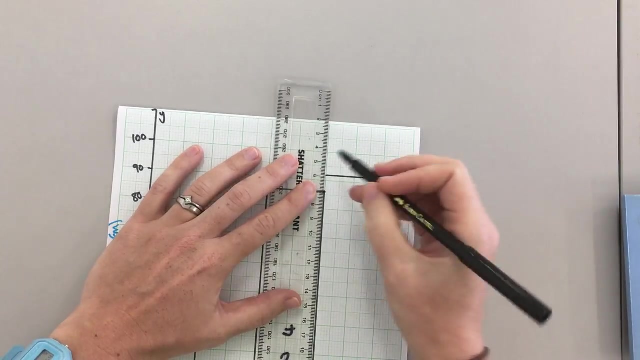 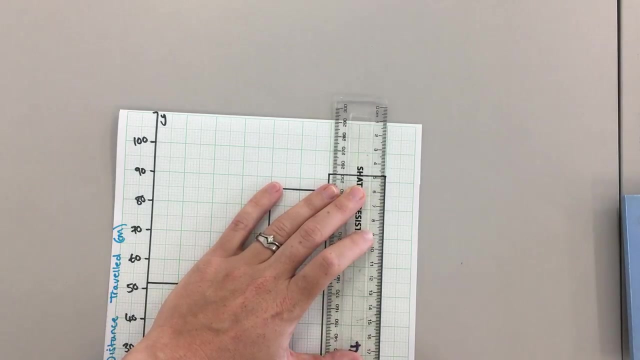 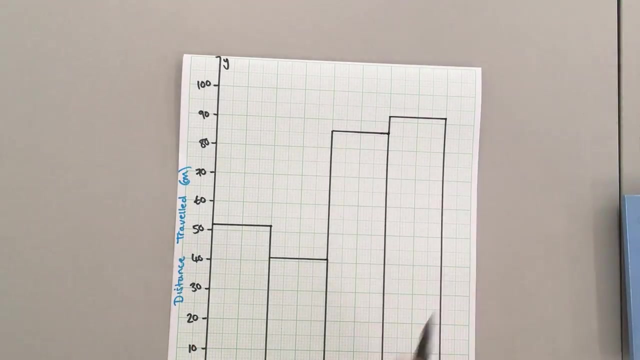 Draw a line across, join it up to my x-axis. Draw a line across, join it up to my x-axis. Wood went up to 86 and then laminate went up to 92. There we go. looks like laminate allows the furthest distance travelled.